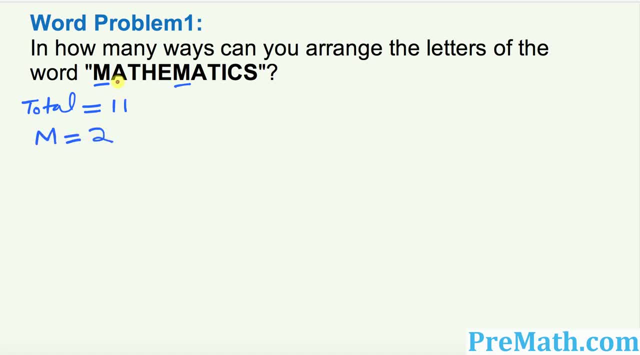 Twice. Put down 2.. Once again, A is repeating again twice. I want you to put down twice. and likewise T is showing up twice. So put down: T equals to what 2.. Next step: I want you to put down total number, which is what 11 with a? 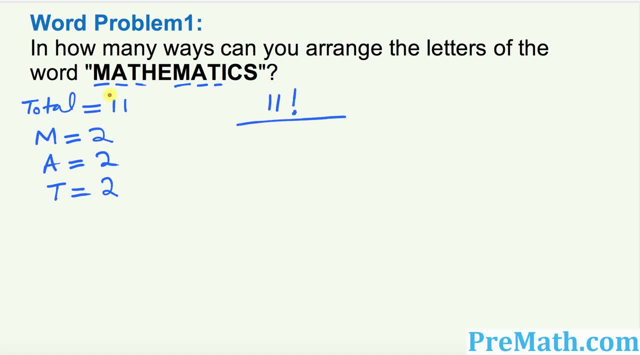 factorial sign divided by C, How many of them are repeating A, M and T. So M is repeating twice. So you put down for M 2 factorial for A, 2 factorial again times 2 factorial for T. Now let's go ahead and simplify these factorials and 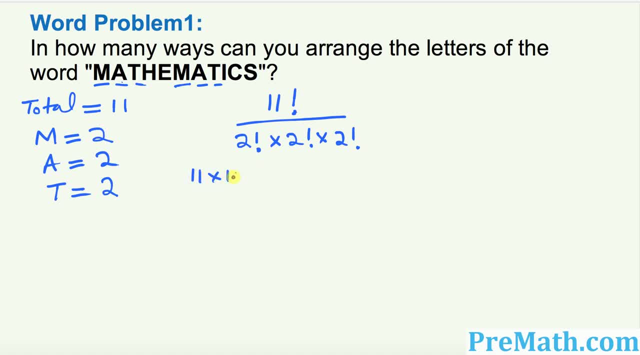 we're going to get our answer. So 11 times 10 times 9 times, 8 times, 7 times, 6 times, 5 times 4 times 3 times 2 times 1 divided by- look at this thing: 2 factorial. by the way, 2 factorial is same as what? 2 times 1, which is same as 2, so I can write. 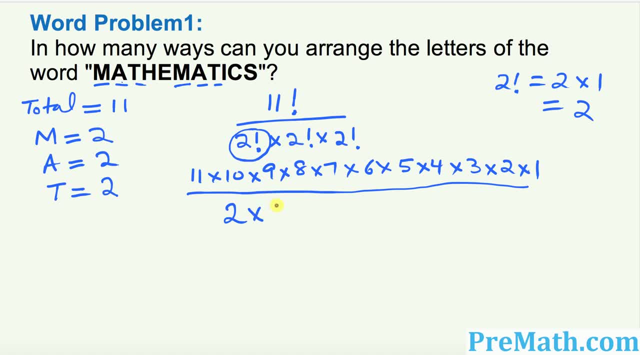 this as a 2. the next 2 factorial could be written as times 2, and then 2 factorial times 2. now what I want you to do is, on the numerator, multiply all these number out, use the calculator. so what is gonna be that one? so that is simply, is gonna give you what: three, nine, nine, one, six, eight. 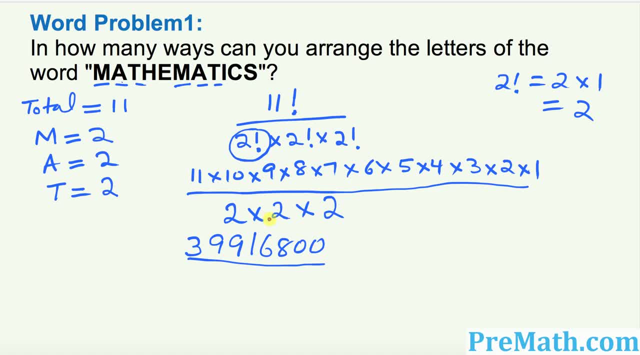 zero. zero divided by 2 times 2 times 2 is 8. let's go ahead and divide these one out. so our complete answer is gonna be: what four, nine, eight, nine, six hundred are. simply, you can put down for the common million nine, eighty nine thousand six hundred and that is. 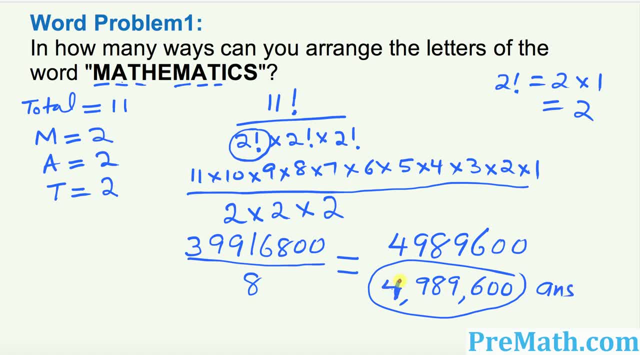 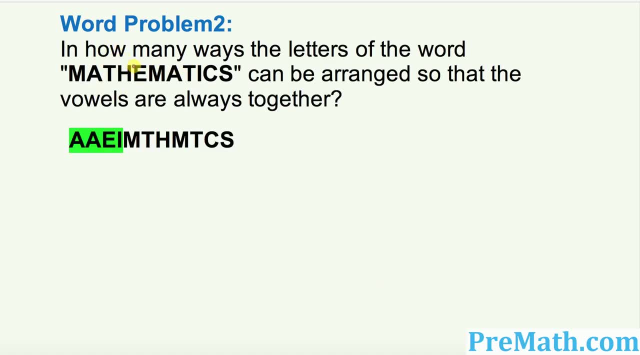 our answer to word problem number one. now let's move on to our word problem number two. in how many ways the letters of the word mathematics can be arranged so that the vowels are always together? so you have to be careful over here. I have already put vowels over here, as you can see, shaded one. 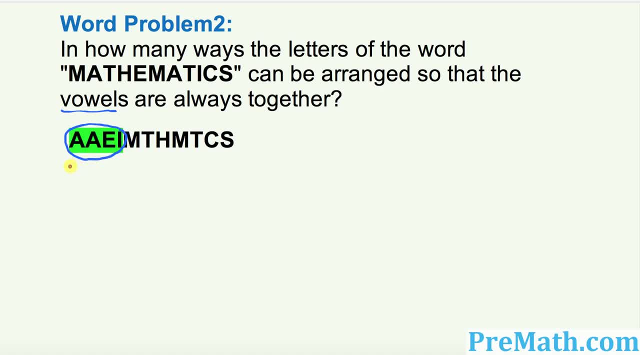 together. so this is just one group. I want to call it vowel group over here, and these are your consonants are now put separately. so the very first thing, again, the way we did before, we want to put down how many total these groups are okay, so that the 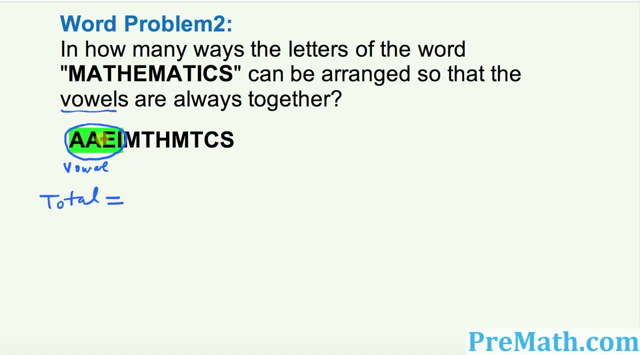 letters. so how many? so this vowel is just one group, so do not look at it, for it is just one. so this is going to be one. M is going to be 2, T, 3, 4, 5, 6, 7 and 8. so we're going to have a 8. now we're going to put it down like this: one over. 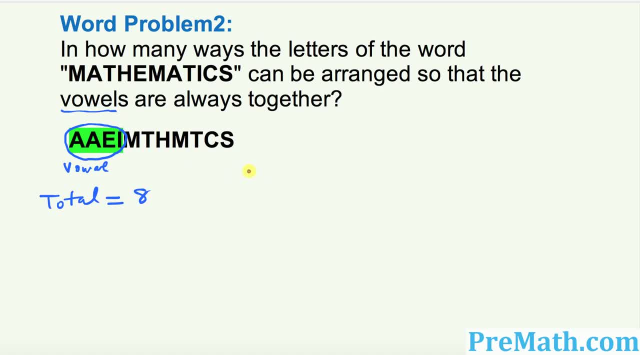 here. our next step is going to be: I want you to put down 8, the total on the top divided by now. ask yourself: are there any num? any of these letters? they are repeating themselves. M is repeating itself and T is repeating itself as well, so that means 2. 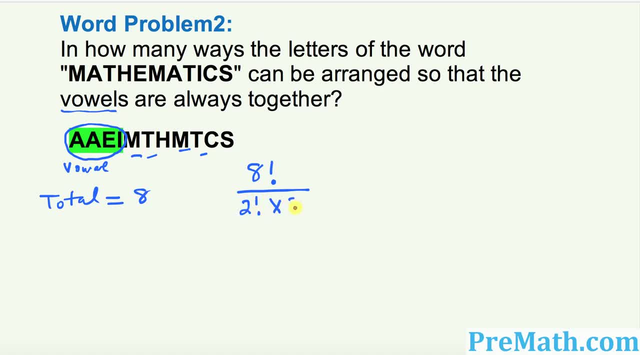 factorial for M times 2. factorial for what T again times now. now you're going to be focusing on vowel group right now. so vowel group has how many letters? inside it has 4. I want you to put down 4 factorial divided by within that group. do you see any vowel that repeats itself? yes, a, so a. 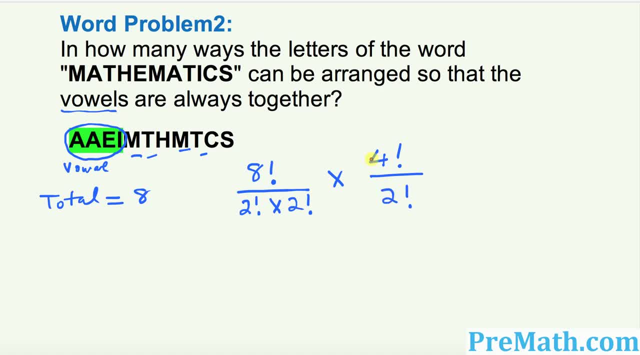 is repeating twice, so I'm going to put down 2 factorial. so in other words, right now, over here, right now, you can see that one. so this over here, this part, belongs to what vowel group? So now, once again, the next step is: I want you to go ahead and simplify this. 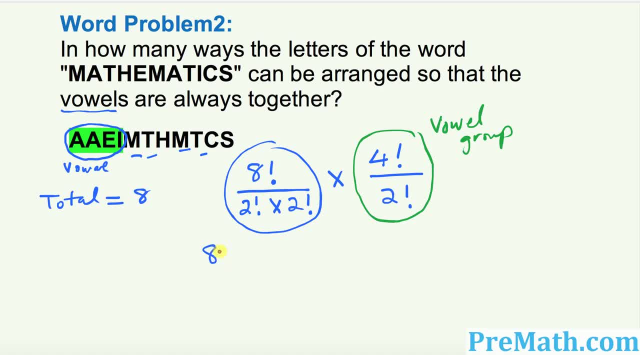 part first. so 8 factorial could be written as 8 x 7, x, 6, x, 5 x, 4 x, 3 x, 2 x 1 divided by 2 factorial could be written as x 2x 2 and then x 10's and we divide by 2. 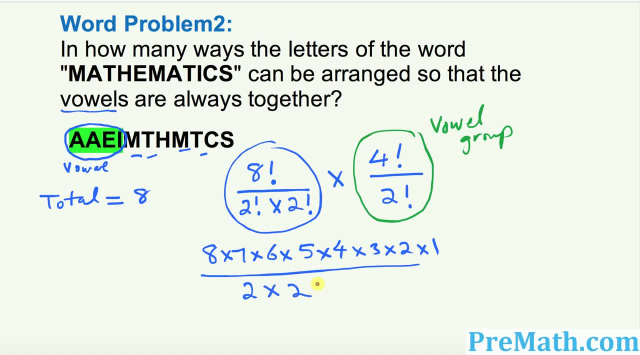 factorial could be written as 2 times 2, and then x 11 times 2 times Wonder, 1.. then times over here and then on this one over here. vowel group is what four factorial could be written as: what four times three times two times one divided. 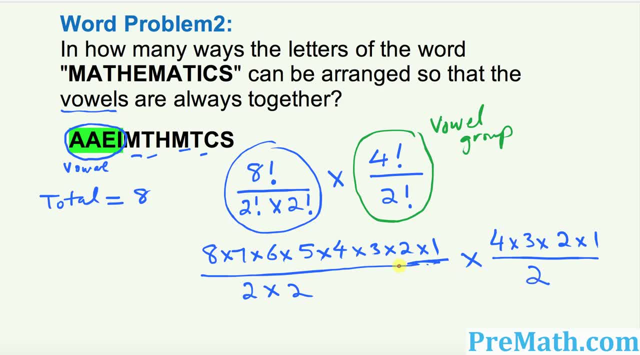 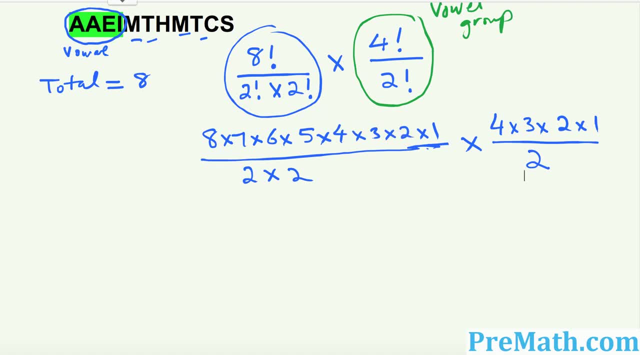 by two. factorial is two, right now, over here, once you simplify this part over here, everything over here, the one that circle, must multiply and divided by two times two is four. we're gonna get what? we're gonna get one, zero, zero, eight, zero and then times. now let's take care of this part over here. four times three. 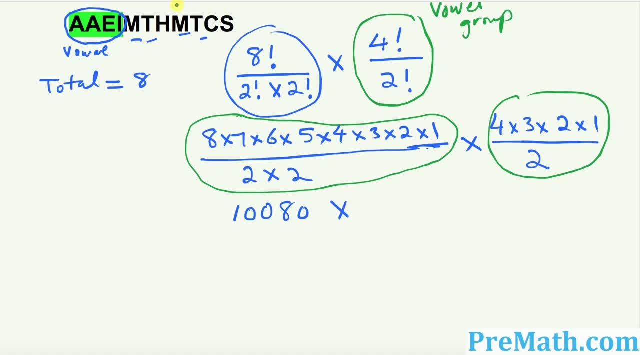 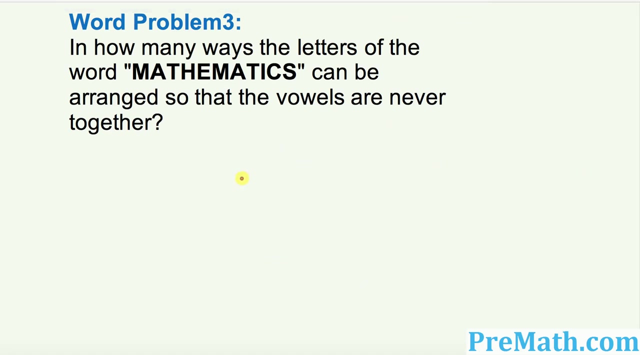 times two times one, divided by two, that is gonna give you our. obviously that's gonna give you twelve. go ahead and multiply them out and that is gonna give you one, two zero, nine six zero. that means one twenty thousand nine hundred and sixty, and that is our answer. now let's move on to our example three. 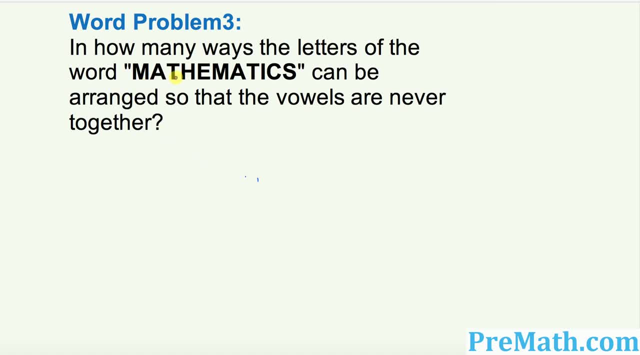 which is called what problem number three. in how many ways do we know what problem number three is and how many ways do we know the letter of the word mathematics can be arranged so that the vowels are never together. so be careful: never together is same as writing what. so let me just go. 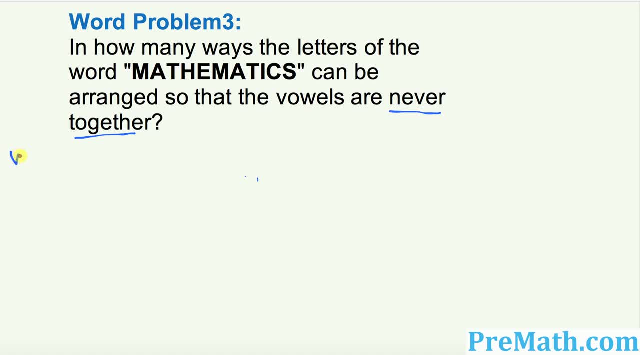 ahead and explain it to you. when they are, vowels never together is same as the total number of these vowels, these ways you can write mathematics. go ahead and write down total number of ways minus and then the vowels, the total number of ways the vowels are together. so vowels are together. 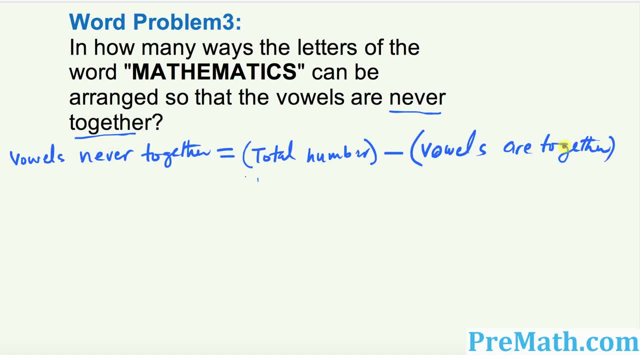 they are together. so if you look at this thing, total number- that was our word problem, that was our word problem number one and this was our word problem number two. we just took care of that one. so let's go ahead and do that one when we say total number. 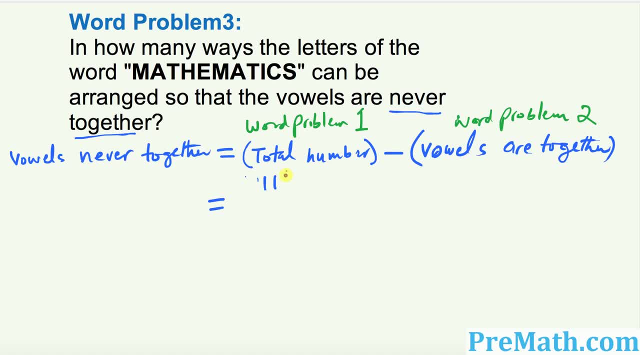 means was what? oh, two times four. because what we did was I did the two terms, which were a, two, pass equal to two, and if I take five by two, I will take it equal to four, and if I fairly, this affects just how many times. fifty times, fifty times, I'll like ten times, twice, that's. 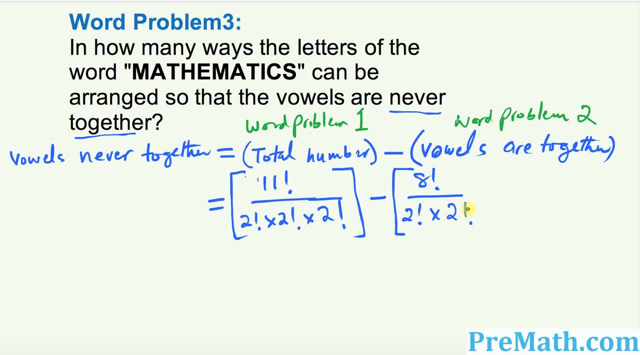 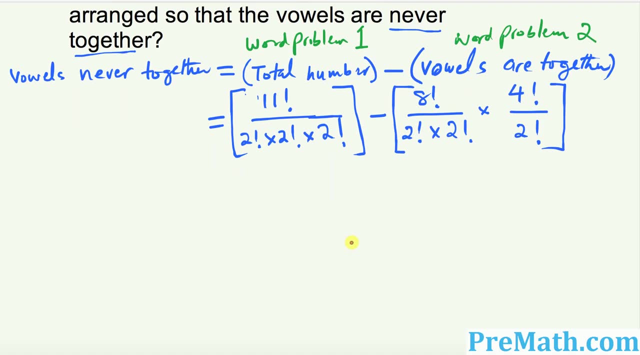 gonna be twelve. so now, at least recommended by me, but in this equation a whole to us factorials times, we did four factorial over two factorial. if you look back on those word problems number one and two, you can see that one. now what we're going to do is right now. 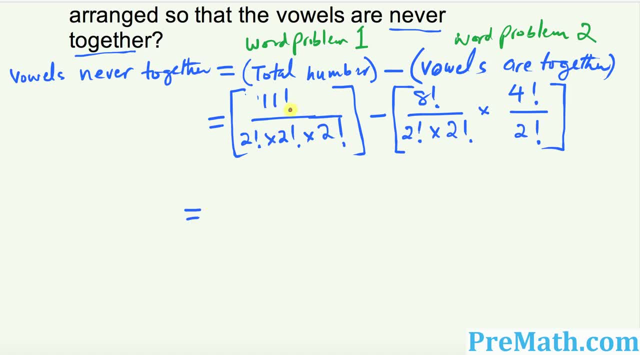 we already found the answer to word problem number one. that was, how much? four, nine, eighty, nine, six hundred, and then minus this portion, we found out one hundred and twenty thousand nine hundred. and what sixty. we're going to just subtract that one and we're going to see what we got. we got how? 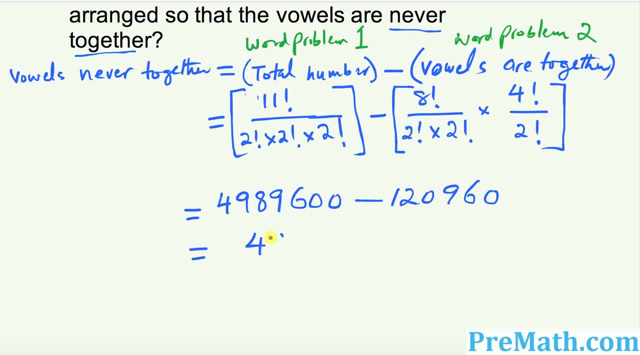 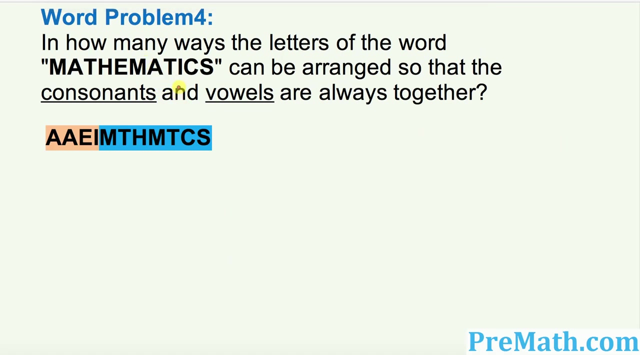 much. four, eight, six, eight, six, forty, and that is your answer. these are many different ways we are going to do that one. and finally, now that's the last problem of this video, is what? problem number four, in how many ways to tote the letters of the word? 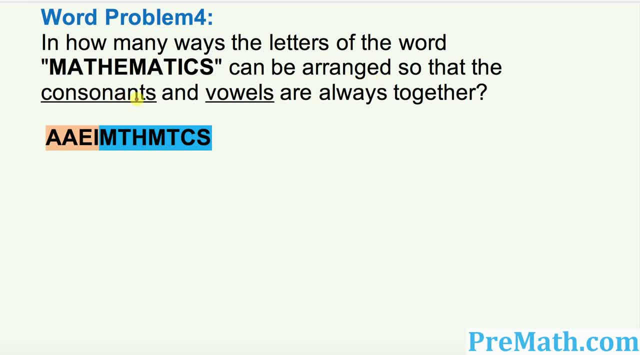 mathematics can be arranged so that the consonants and vowels are always together. so now, as you can see, there are two shaded parts. I have already put them different shade. that is your group one, that is I'm going to be calling vowels, and this part we will be calling what? kons Ohio. 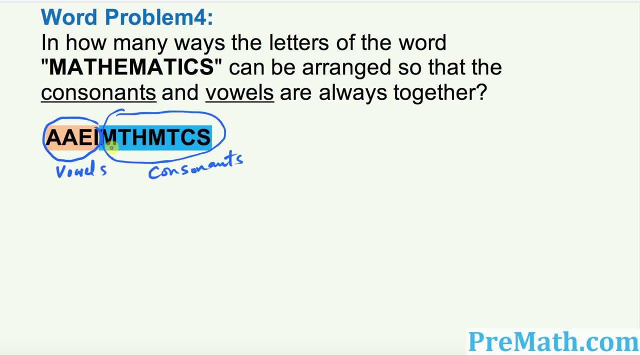 part over here. so we have a two entities, two groups. so when you're going to start off, you're going to just simply put down only two factorial, because we have two groups. times now we're going to be focusing on our vowel group. how many letters are in vowel group? there are four of them. I'm going to put down four. 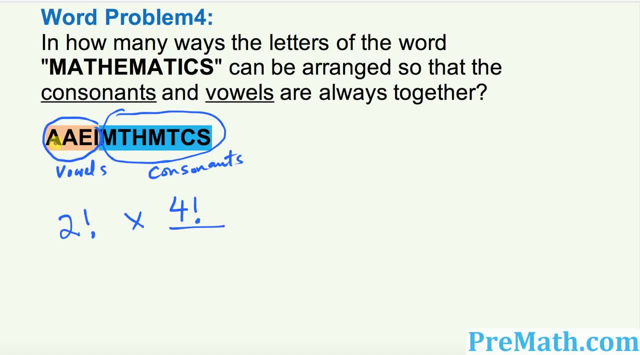 factorials and ask yourself: are there any letters that repeat themselves? yes, a repeats how many times? two times. so I'm going to put down two factorials for a and then times over here. so I want you to put down times over here. look at the consonants, consonants. you see how many consonants are over there, there, how many. 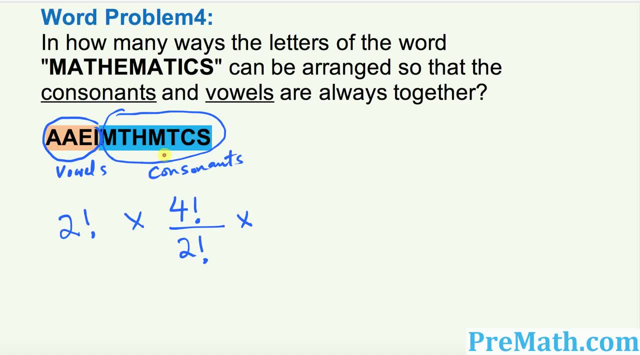 count them: one, two, three, four, five, six, seven, eight, nine, ten, eleven, eleven, eleven, four, five, six, seven. I want you to put down seven factorial right up here and again. ask yourself: are there any letters that they are repeating themselves? yes, of course, M and T. they are repeating twice. so for M you put down two. 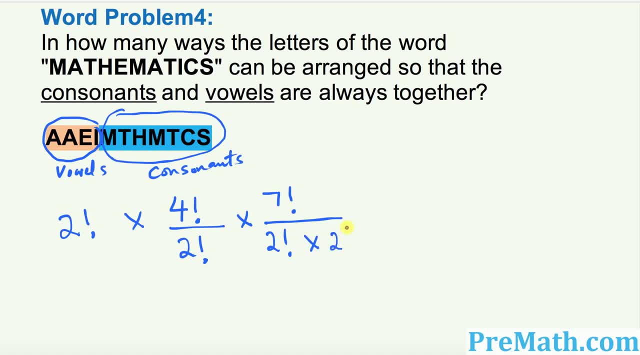 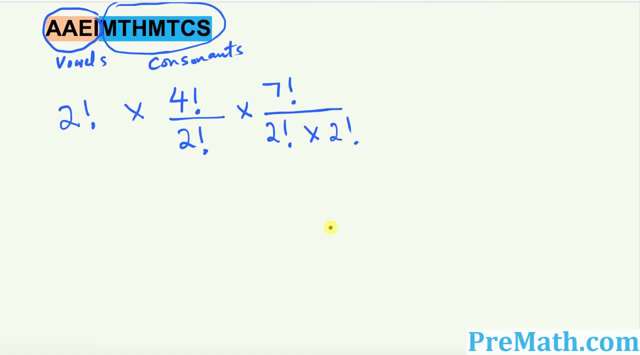 factorial times. two factorial for T, and now we're going to go ahead and simplify these problems over here. not bad. so once again, I just want to make sure this part is two factorial, for both of them separate entities, vowels and consonants. and this is for what? so? 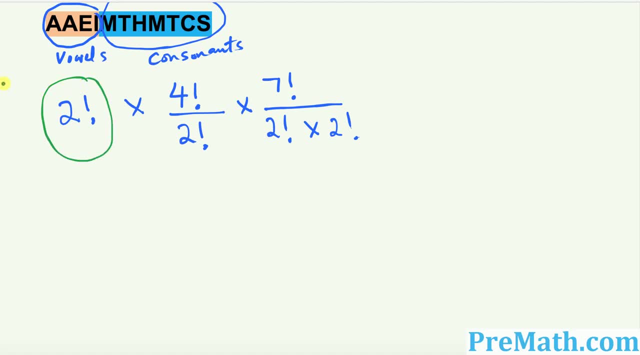 this is for. this is going to be for both vowels and consonant. this is going to be for what vowels and this thing is going to be for what consonants. okay, so just keep in your mind. right now, let's go ahead and simplify. two factorial is same as two times four. factorial could be written as: 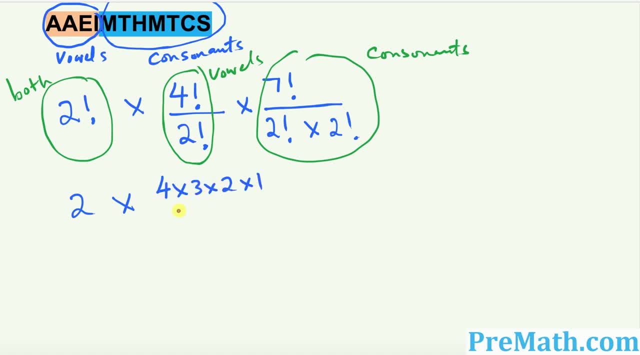 four times three times two times one. divided by two, factorial is same as two times seven factorial could be written as 7, 6, 5, 4, 3, 2, 1 divided by two, two factorial is same as two times two factorial is same as two. let's go ahead and now simplify. 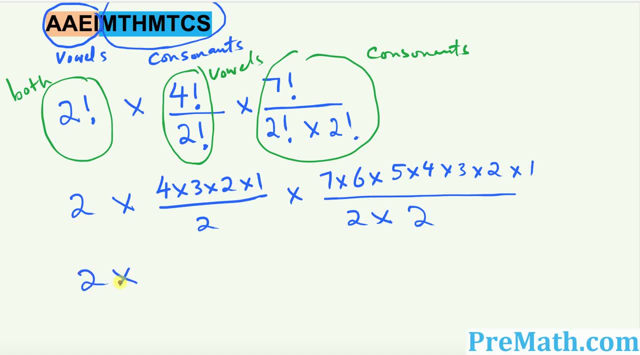 these one, so this is two times. once you simplify this part over here, that is gonna give you how much that's gonna give you 12 times. if you simplify this whole thing, that is gonna give you 1260. and when you multiply 2 times 12 times 1260, that's going to give you 30, 240 and that is your. 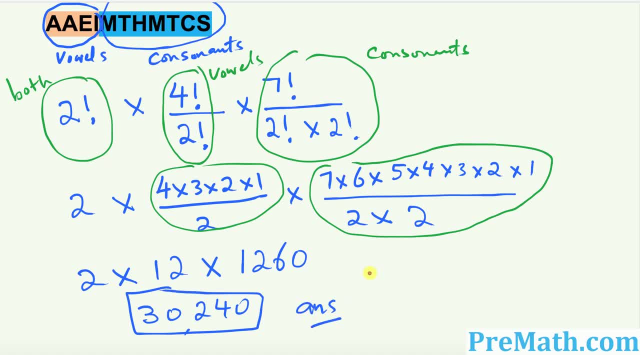 complete answer. thanks for watching, bye.